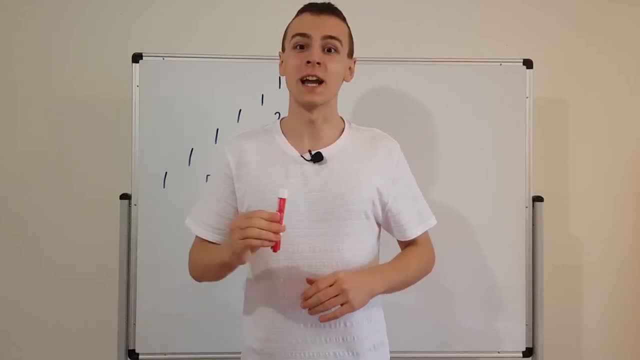 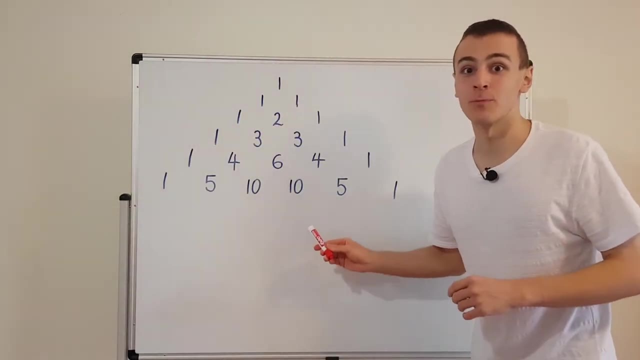 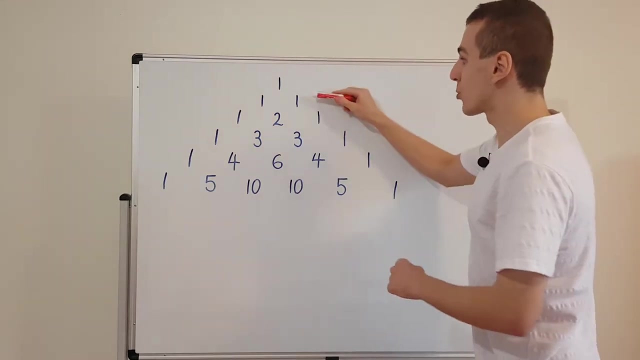 Let's discover where the powers of 11 are hidden in Pascal's triangle. Over here I've drawn the first five rows of Pascal's triangle. By convention, this one over here is defined to be row zero. So this is row one, row two, row three, four and five, And we could keep going on and on forever. 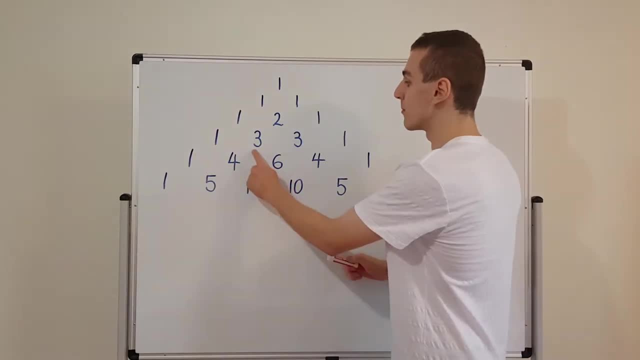 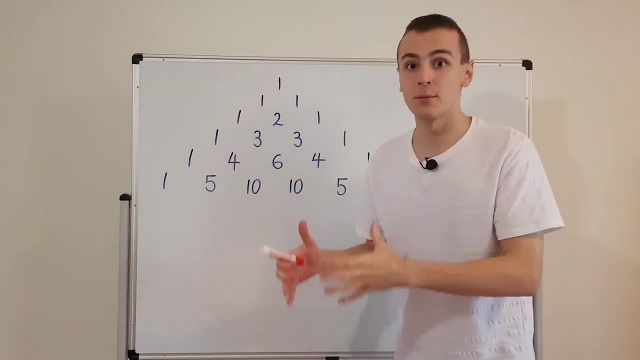 One pattern I want you to notice is that if you take the sum of two adjacent numbers, that actually gives the number that's directly below, And that's the pattern that's used to construct Pascal's triangle. You start with these guys in the top, these two ones combined to give 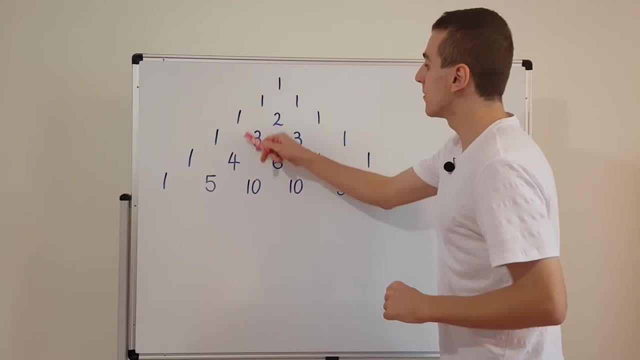 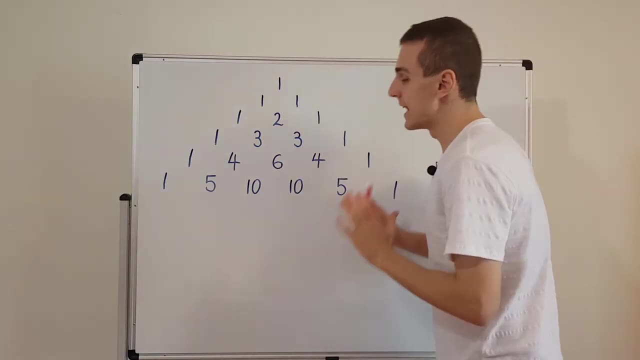 a two, and then each of these guys combined together to give the number that is directly below. For example, three and three are six, six and four are ten. Now what I want to do is I want to actually discover where the powers of 11 are hidden in this triangle. If we read each of the 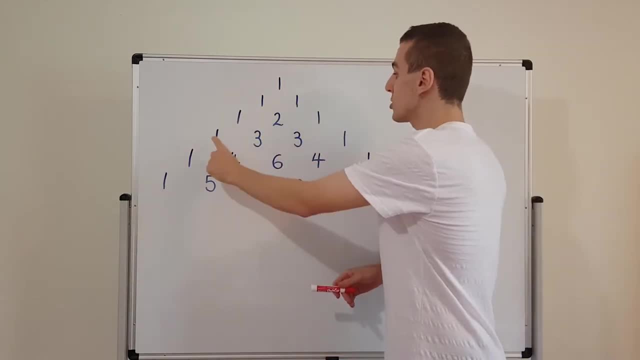 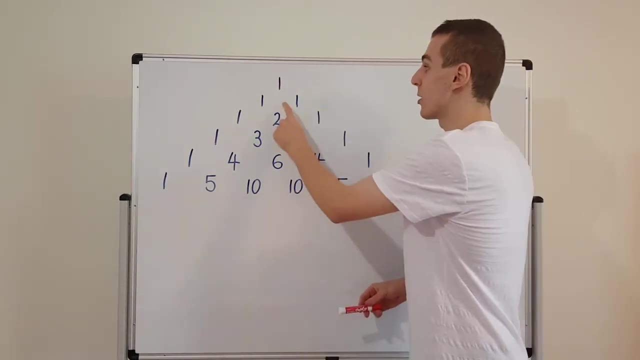 digits or each of the numbers, we're going to be able to find out where the powers of 11 are. So we take the numbers in the rows and we can actually discover that these guys are the powers of 11.. 11 to the power of zero is 1.. 11 to the power of 1 is 11.. 11 squared is 121.. And this 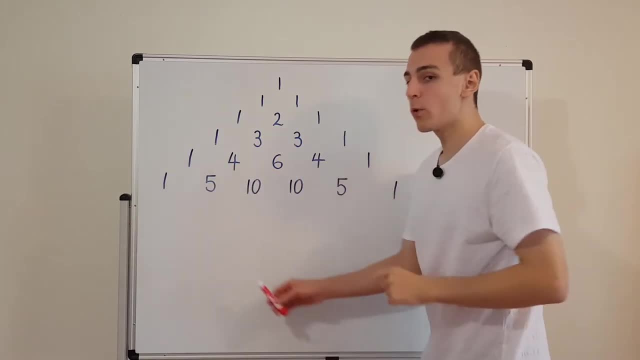 over here is 11 cubed 11 to the power of 4.. But what about? over here? We have 10 and 10.. We'll get to that in a moment. Let's write down what we've noticed so far. So this zero throw corresponds to 11 to the power of 5.. 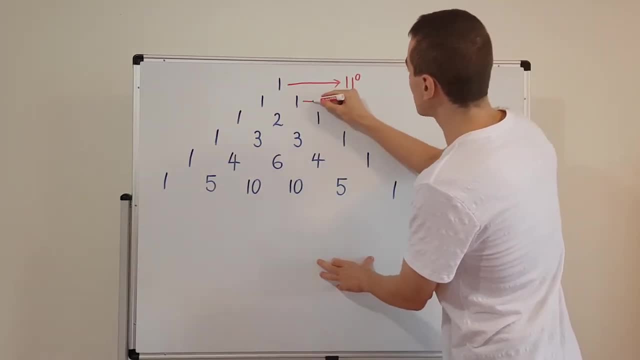 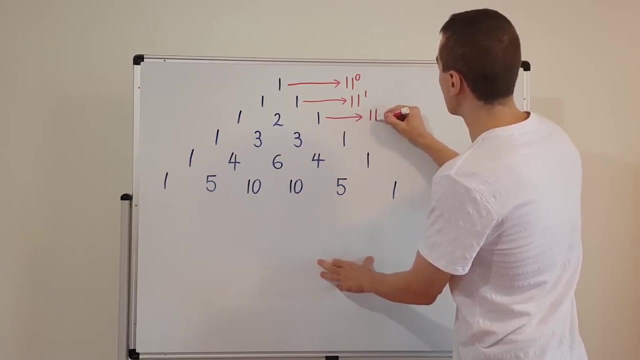 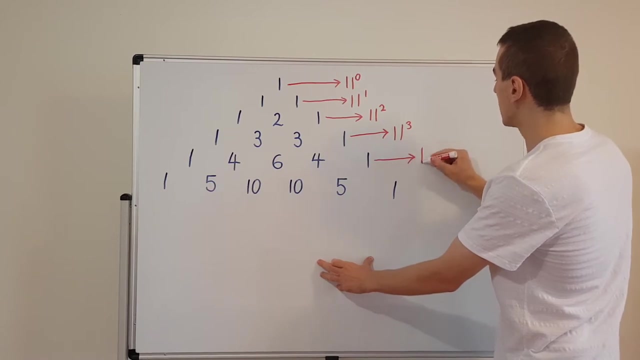 power of 0.. This first row corresponds to 11 to the power of 1.. This second row corresponds to 11 squared. Over here we have 11 cubed, and over here we have 11 to the power of 4.. So how are we? 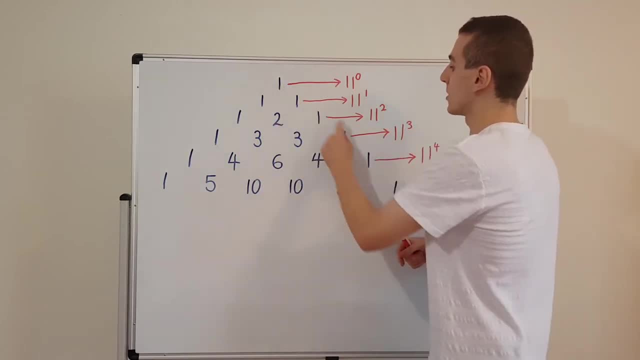 actually constructing these guys. The 1 over here, this 1 is always the 1's digit, and the 1 away from the 1's digit is the 10's digit. And then we have the 100's digit, thousands, and then 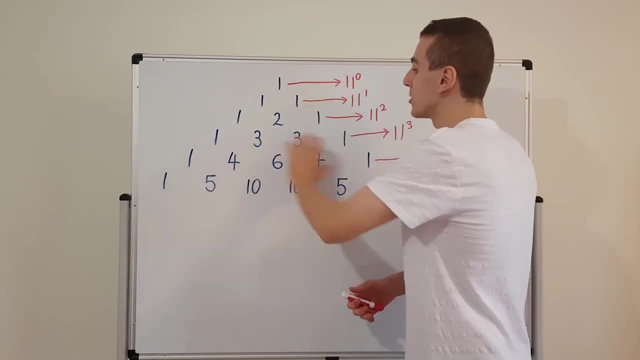 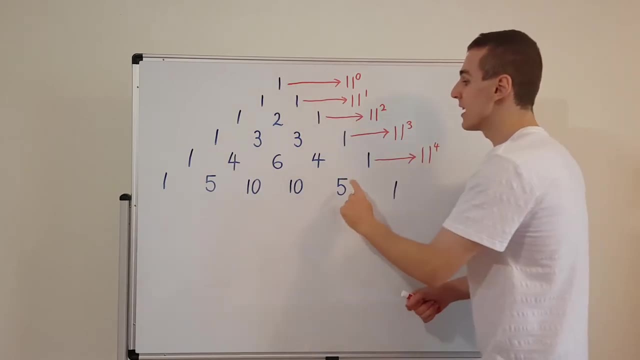 10 thousands and hundreds of thousands. So that is actually the pattern that we can notice over here. The digit that's the furthest to the right represents how many 1's we have, Then we have how many 10's we have, and then there's how many hundreds and then how many thousands. So I'll 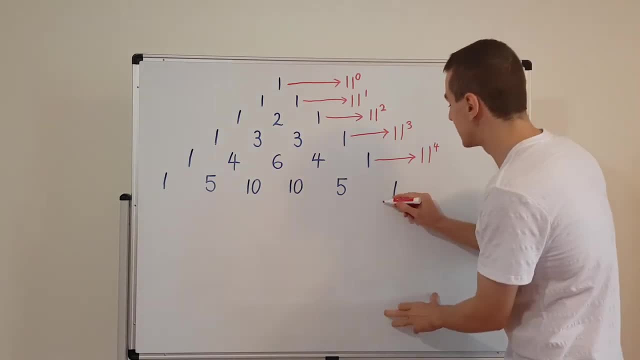 write this out explicitly. What this guy over here is saying is: we have 1 times 10 to the 0.. And 10 to the 0 is 1.. This guy over here it's saying: we have 5 times 10 to the 1, right 10 to. 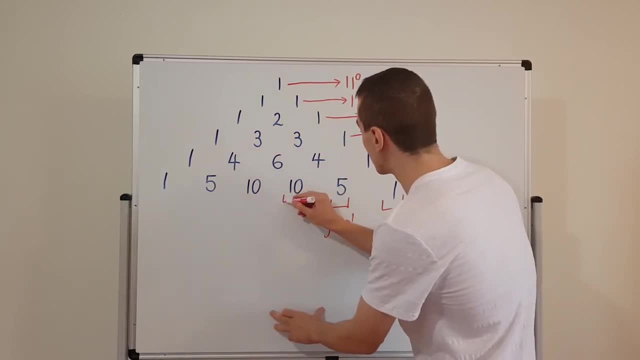 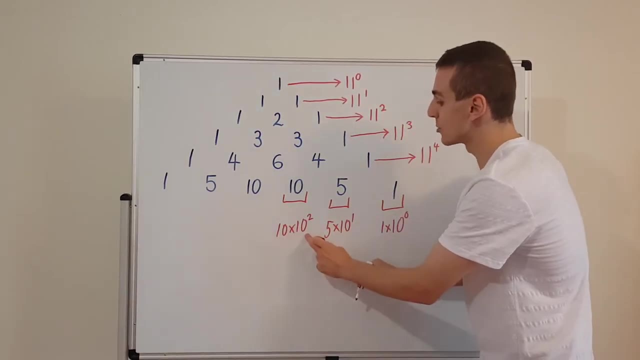 the 1 is 10.. This is the 10's digit. Over here we have 10 times 10 to the 2.. So we have 10 hundreds. And what's 10 hundreds? Well, 10 times 10 to the 2 is 10 to the 3,, which is a thousand. 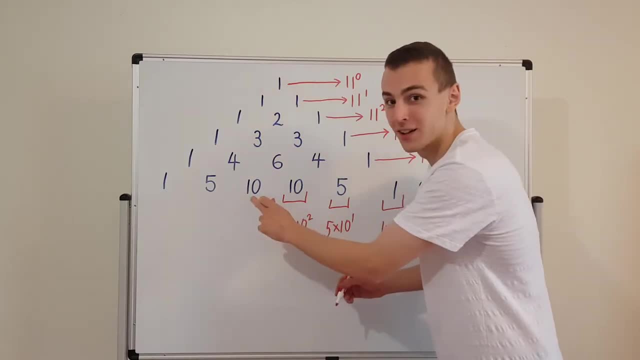 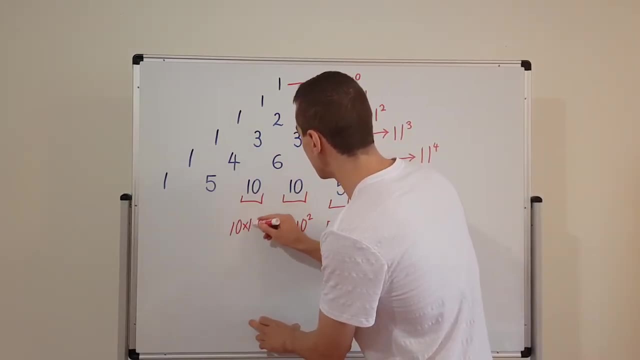 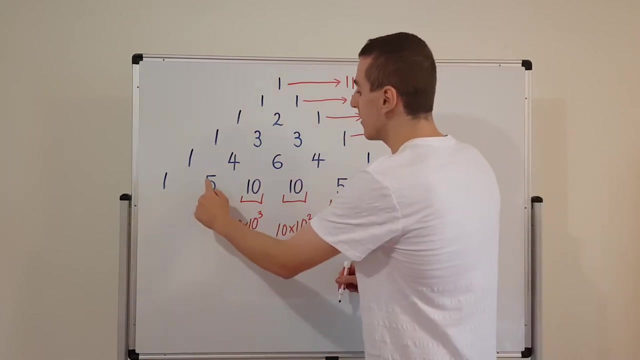 So what we're actually going to end up doing is carrying 1 over to the other digit. So what about this one over here? This is 10 times 10 to the 3, right, This is the thousands digit. We have 1, 10, 100,, 1000.. Now we have 10,000. This over here is 5 times. 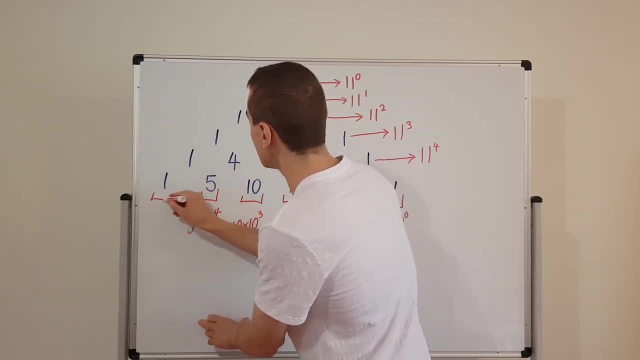 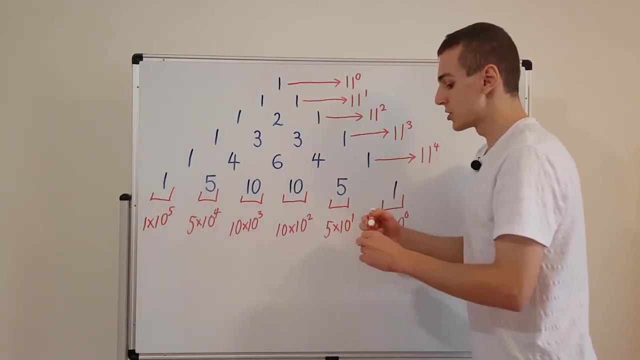 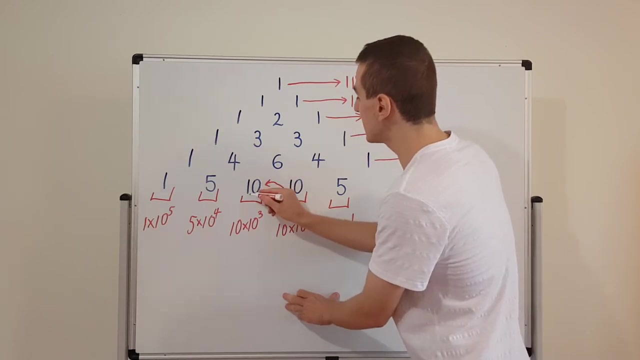 10,000, which is 10 to the 4.. And finally we have 1 times 10 to the 5., And this is 100,000.. So let's do the carrying over And see what we get. So if we carry 1 over to here and we also carry this 1 over to here, 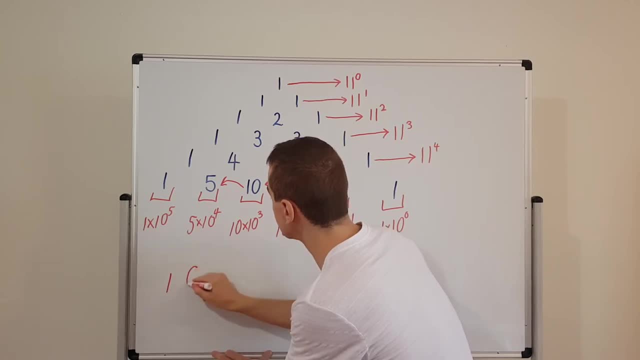 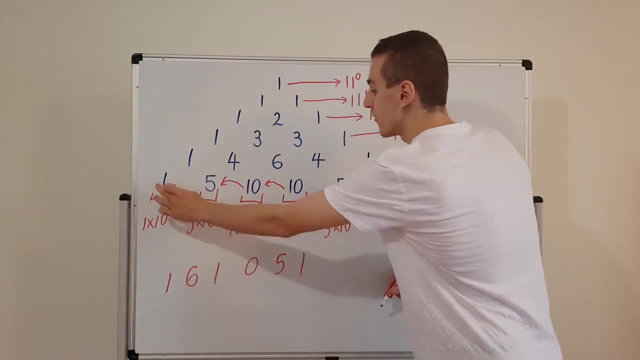 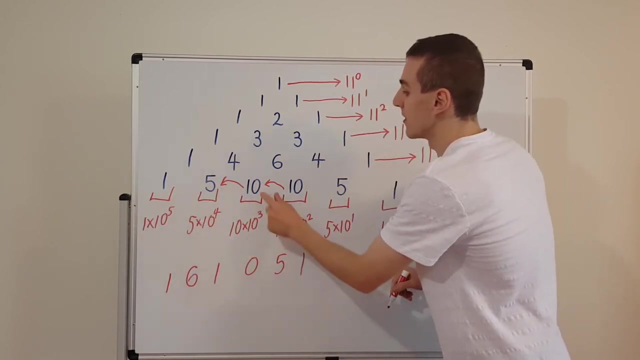 that's going to give us 1,, 6,, 1, 0,, 5, 1, right, That's what this final row is actually telling us. We get a 1 over here. We get a 5 plus 1,, which is 6.. Then we get a 0 plus 1,, which is 1.. And over. 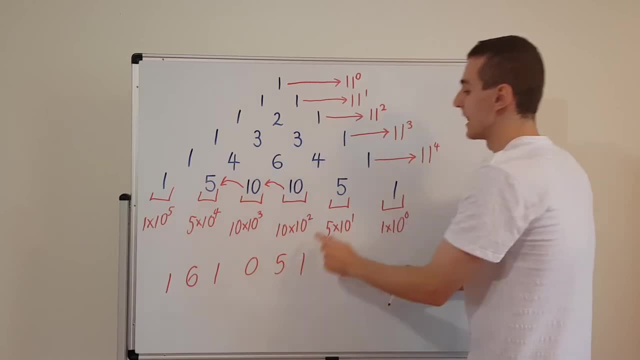 here. this 1 over here is 10 to the 3, which is 10 to the 4. And finally we have 10 times 10 to the 5. 1 gets carried over, so we just have 0. And then we're left with 5 and 1.. So what we get is: